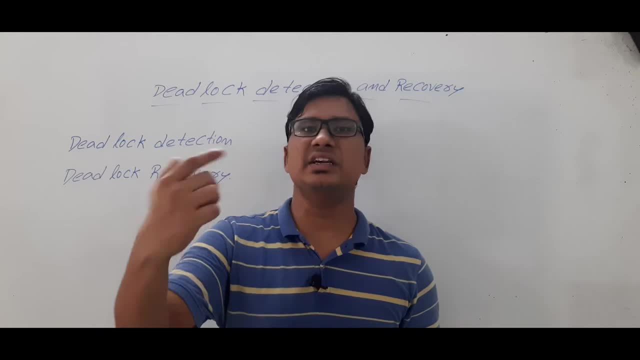 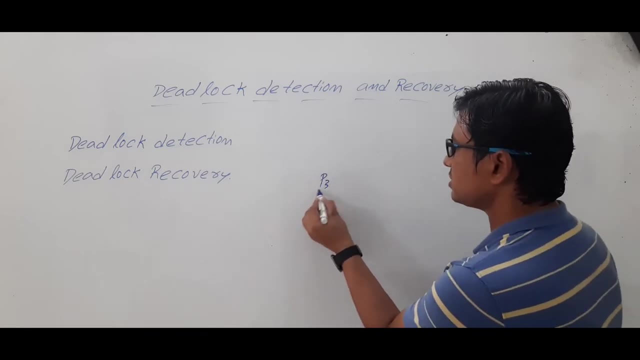 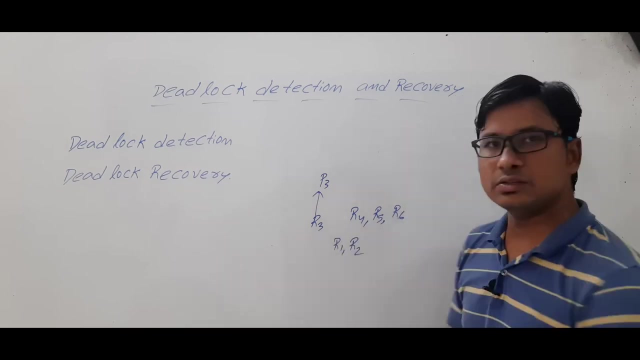 we have kept is that if a process is requesting for resource R3. Let's take that process. P3 is there, Has requested the resource R3 and it has been allocated. Now the next request can be either R4 or R5 or R6. But it cannot request R1, R2.. This is one restriction, or another kind of restriction. 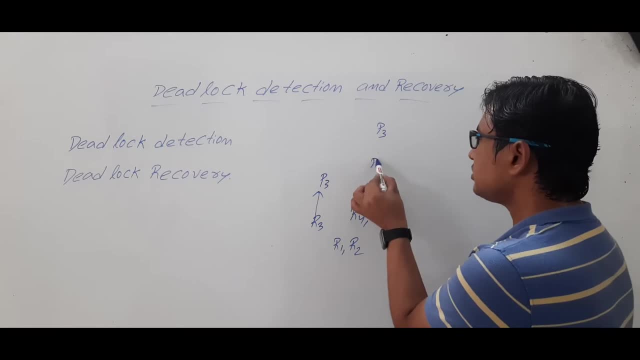 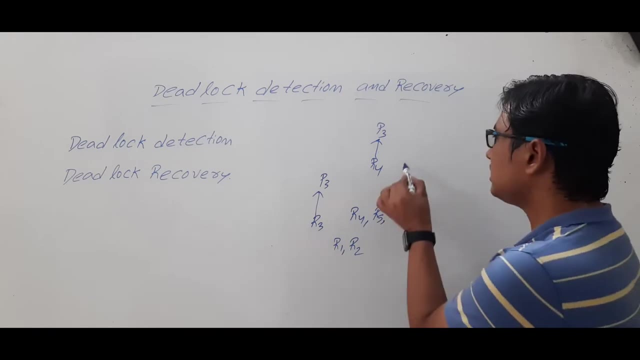 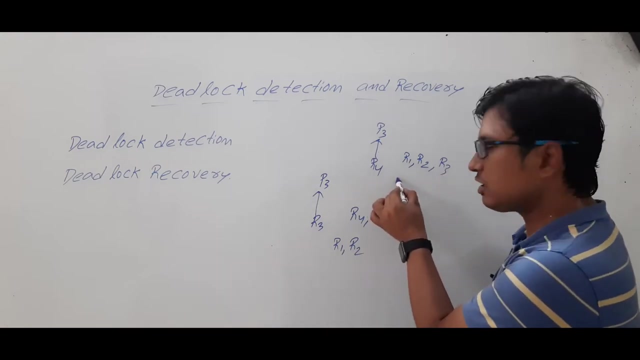 is that? let's take the process. P3 has requested for the resource R4 and it has been allocated. Now the request is that, or the restriction is that it can request for resource R1,, R2, resource R3. But it cannot request for resource number 5, resource number 6.. Is it clear, Any one? 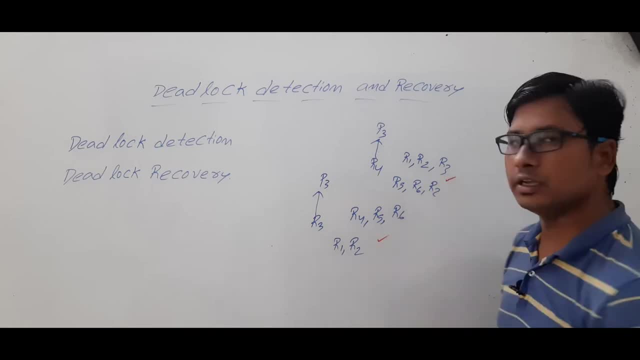 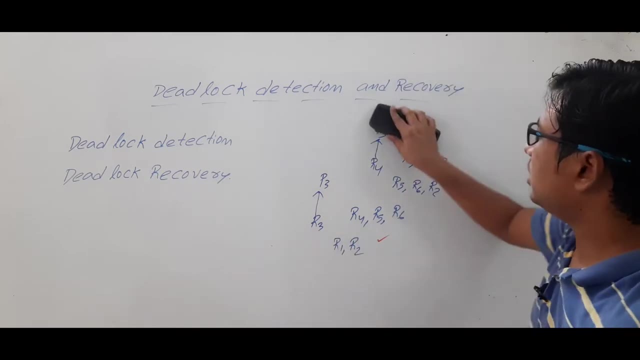 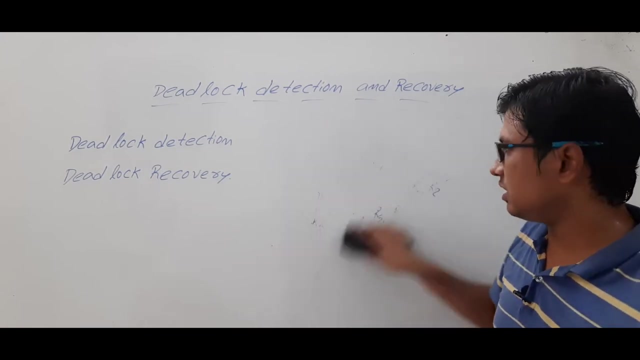 of this restriction, either this one or this one. if you keep, then we can disable the circular wait, which is practically possible. So this is about the deadlock prevention. Then, coming to the deadlock avoidance- we have discussed about the bankers algorithm. The next one is the deadlock detection. 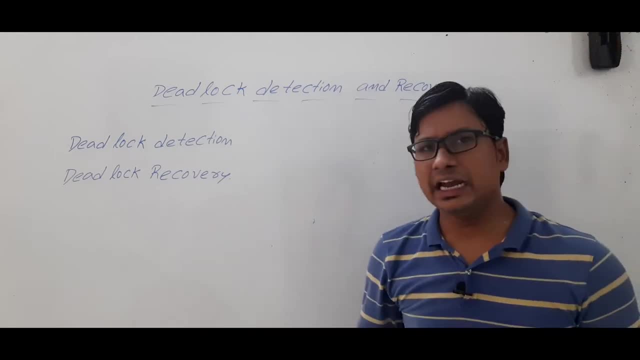 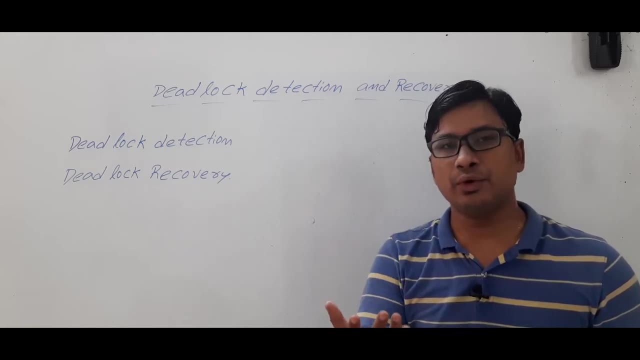 what is the meaning? You will allow the deadlock In deadlock prevention. what you are doing, You are not allowing the deadlock by disabling any one of the necessary condition In deadlock avoidance. while allocating the resource to any process, you are checking whether the system is in safe state. 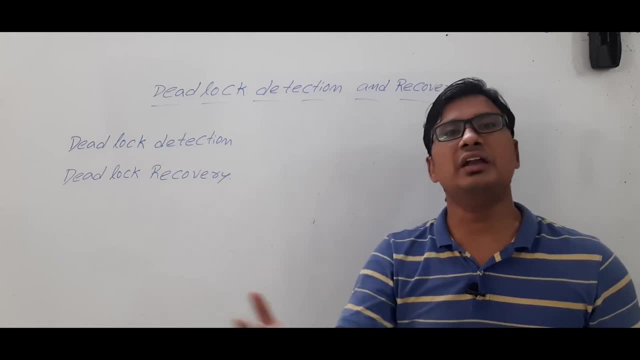 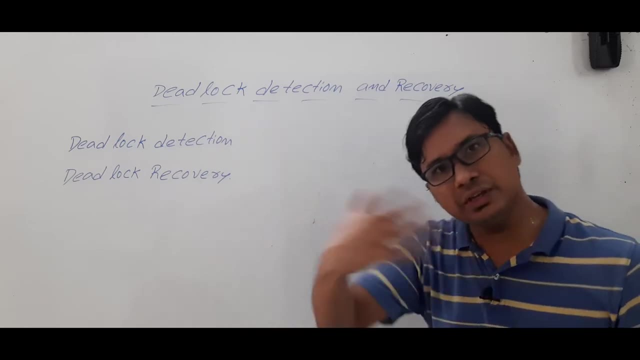 or not. If the system goes to the unsafe state, you will not allocate the resource to the process. Is it clear? Are you able to understand? In coming to the deadlock detection, we will allow the deadlock. Let the deadlock happens, Then we will detect. 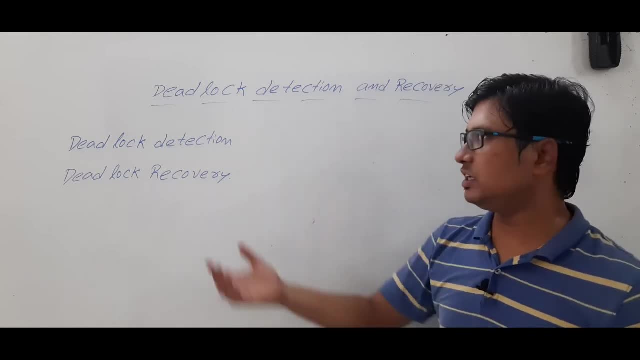 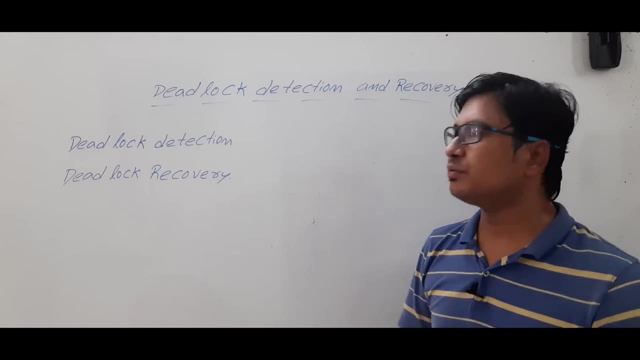 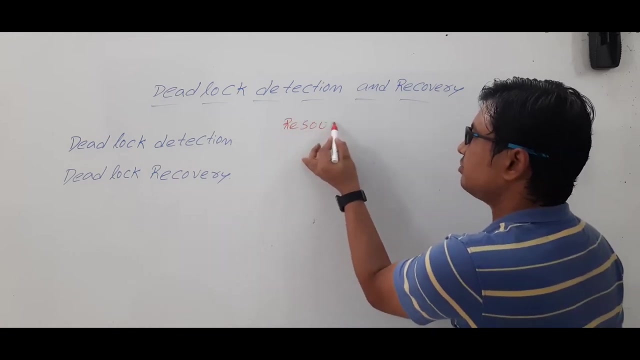 Then we will recover from the deadlock. Is it clear? So we have two phases. One is the deadlock detection and then deadlock recovery. Now let me discuss. how can we detect there is a deadlock? We have already discussed about the resource allocation graph. Is it clear? By looking at the resource? 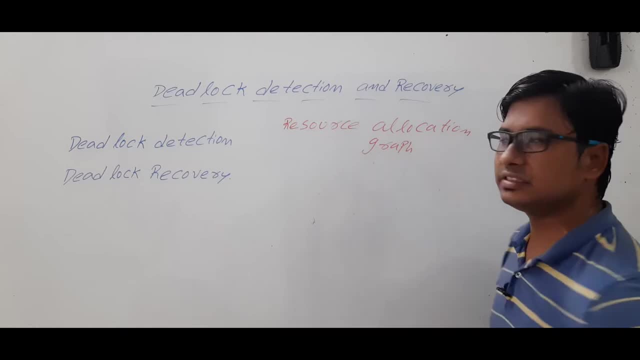 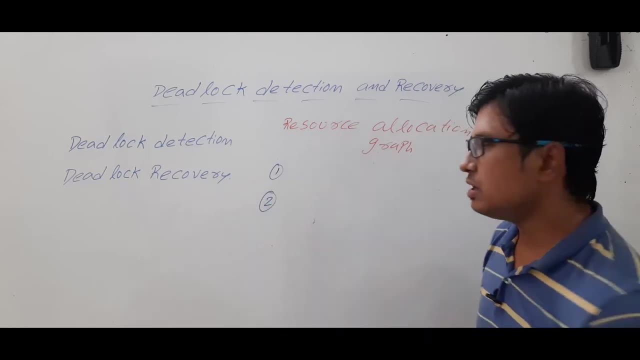 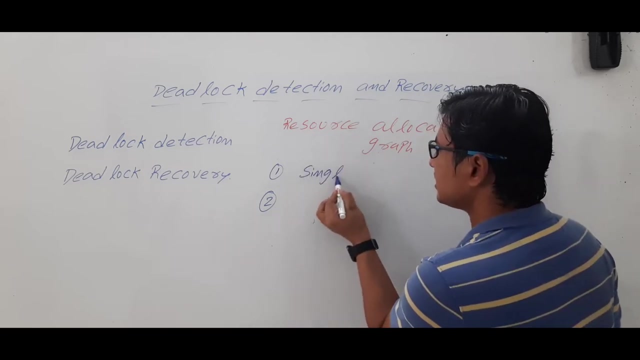 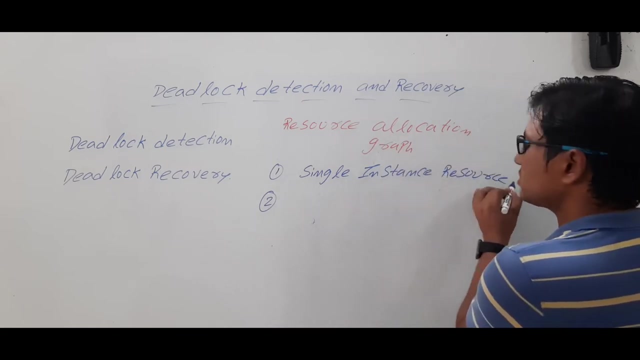 allocation graph. we can find whether there is a deadlock or not. In a resource allocation graph we have two types of vertices. One is the process and another one is the resource. In resource also, we have single instance resource allocation graph. Meaning is that all the resources are. 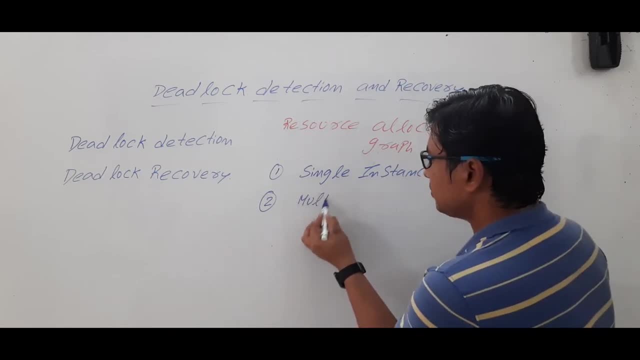 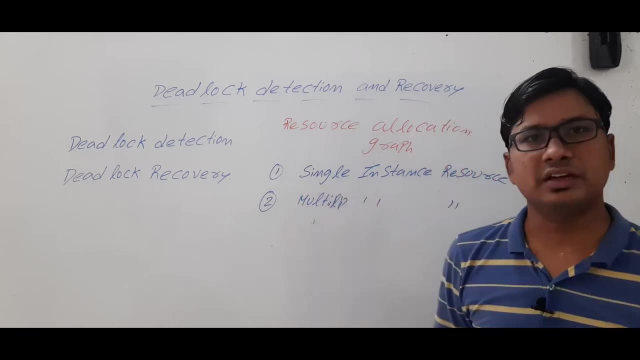 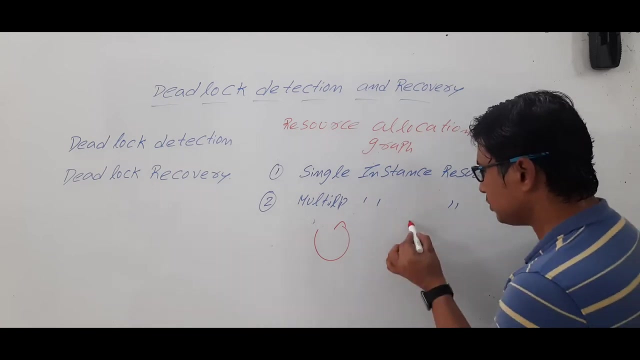 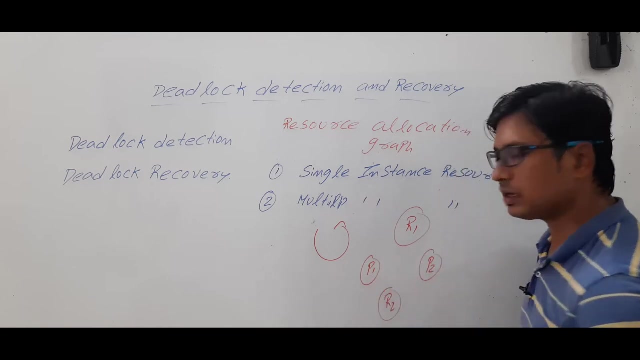 single instance and another one is multiple instance of resource graph. Now, if it is a single instance, we will check whether there is a cycle or not. Let me give an example. You have a resource r1,, you have a process p1,, you have a process p2 and then you have a resource r2.. Usually we will 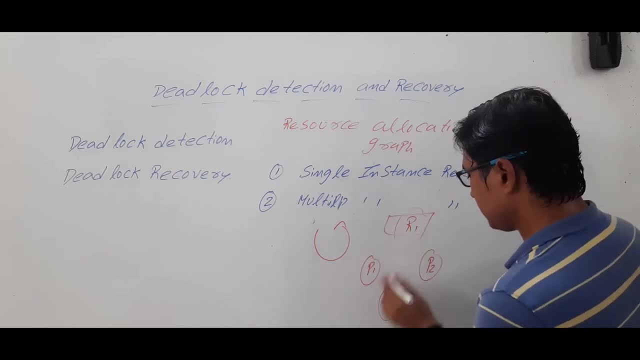 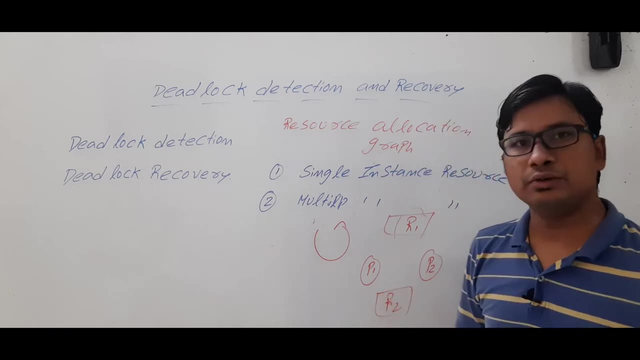 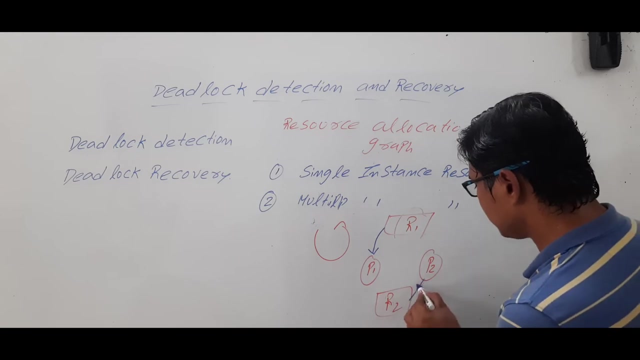 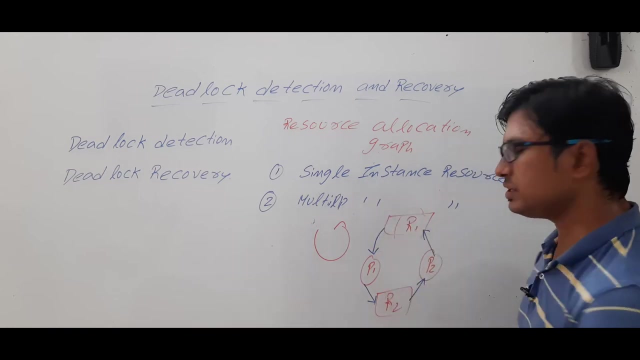 represent resource like this. Let me represent the normal way. Now you have resource r1 and resource r2. both are single instance. Now let's take that one instance of resource r1 is allocated to the process p2.. Now process p1 is requesting for resource r2.. Process p2 is requesting for: 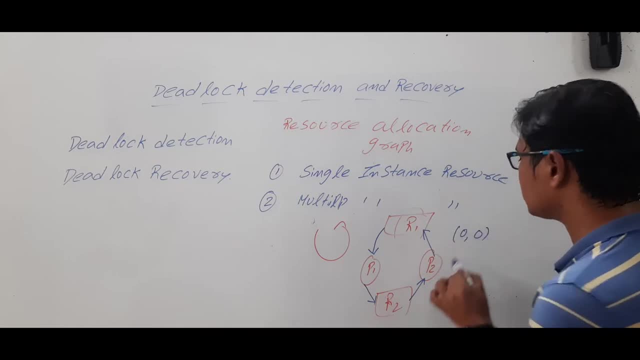 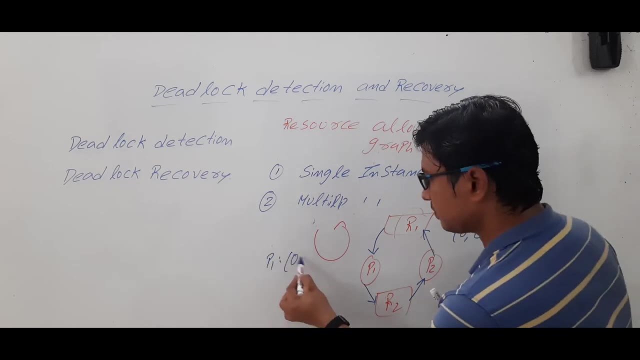 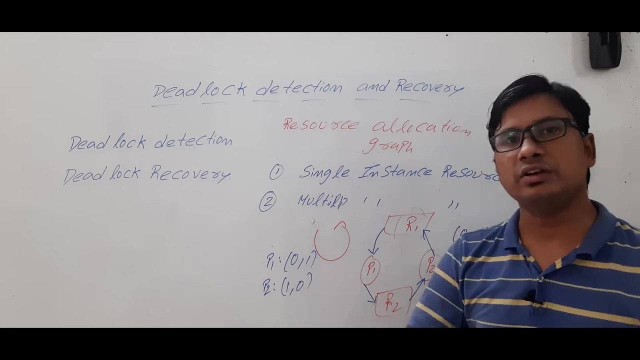 resource r1. Now, the current availability of these resources are 0 and 0, but process p1 requirement is 0 and 1.. It is requesting for the resource r2 and it is not requesting for the resource r1.. Now, Now process P2 is requirement is 1, 0, meaning is that it is requesting for one instance of resource R1, but it is not requesting for the resource R2.. 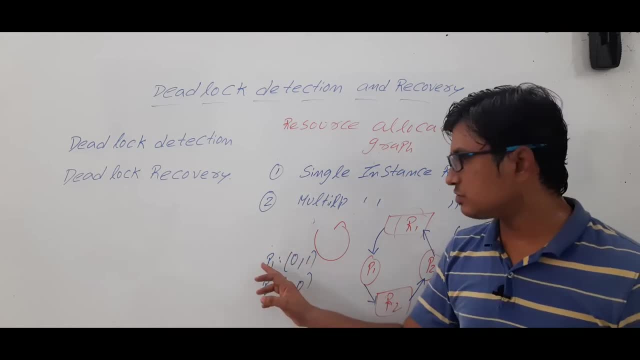 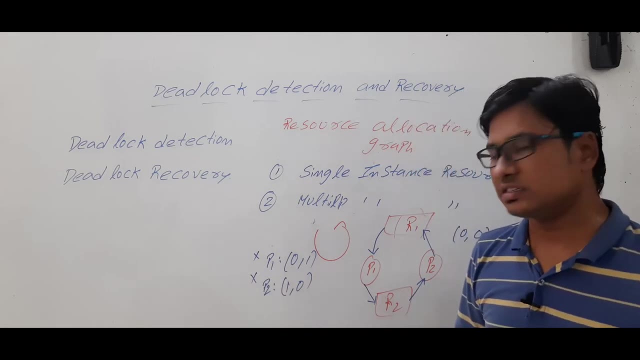 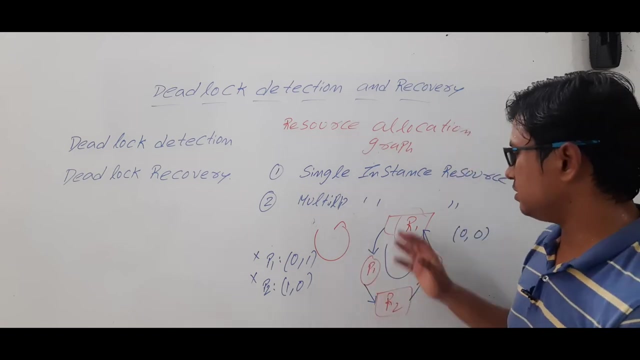 With 0, 0 availability, you cannot satisfy the requirement of process P1 and process P2.. So the system is in, not a safe state or unsafe state. Is it clear or able to understand? And so there is a cycle. whenever there is a cycle in single instance resource allocation graph, we can say that there is a deadlock. 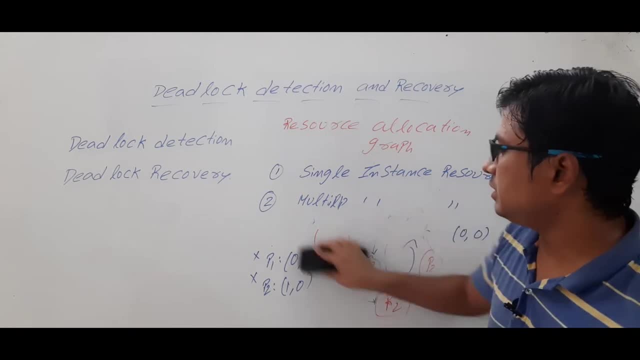 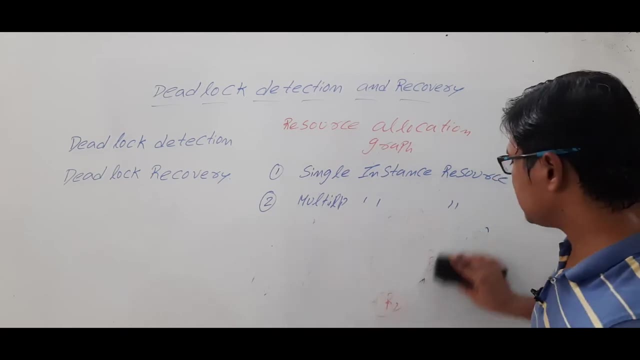 So, like this, we will detect, When it comes to the multiple instance resource allocation graph, we will use the banker's algorithm. whether there is a deadlock or not, We will check it. Can we the system is in safe state or not? 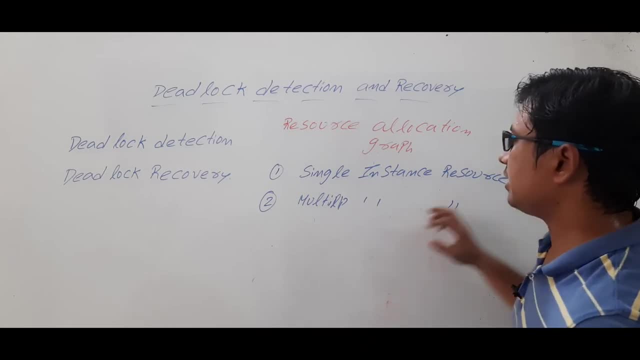 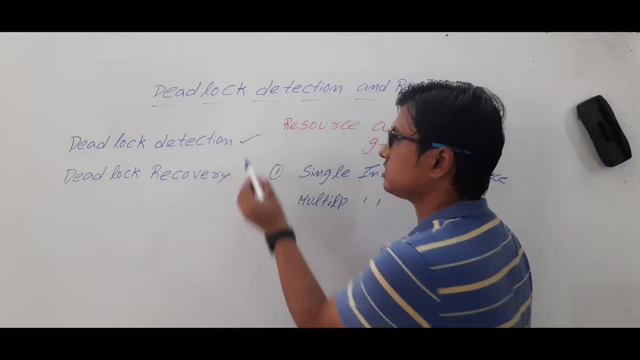 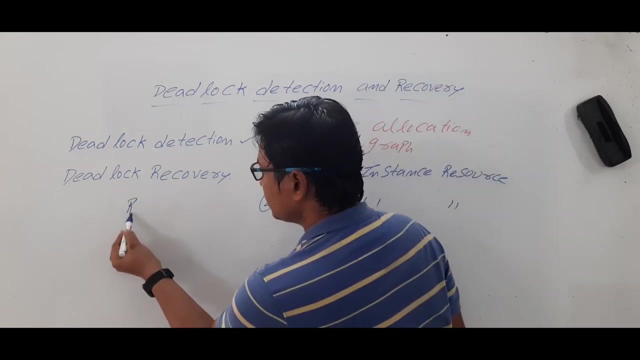 Is it clear. So we will use those mechanisms to find there is a deadlock or not By looking at the resource allocation graph. So we have discussed about the detection. Now we will discuss about the recovery. Now the recovery is with respect to the resources and with respect to the process. 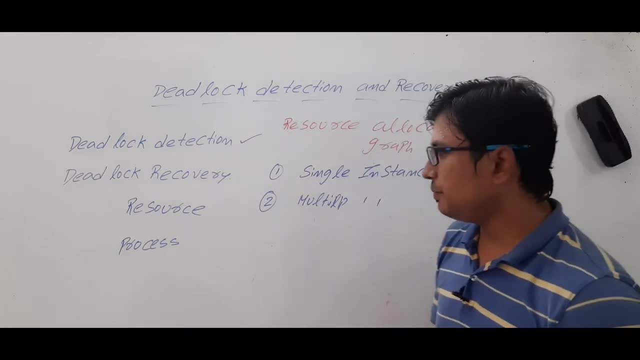 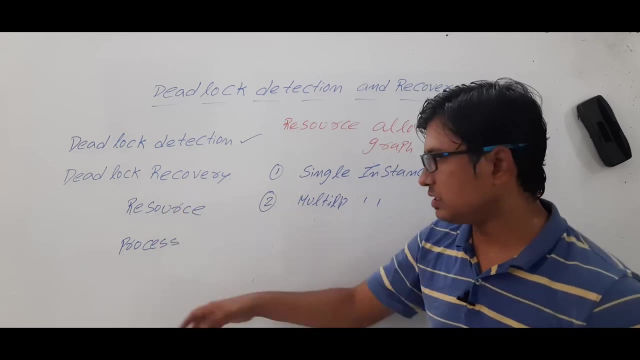 Okay, Now let me discuss with respect to the process. Meaning is that we can recover from the deadlock with the help of the process, with the help of the resource. What is that one is With respect to the process is kill Any one process. 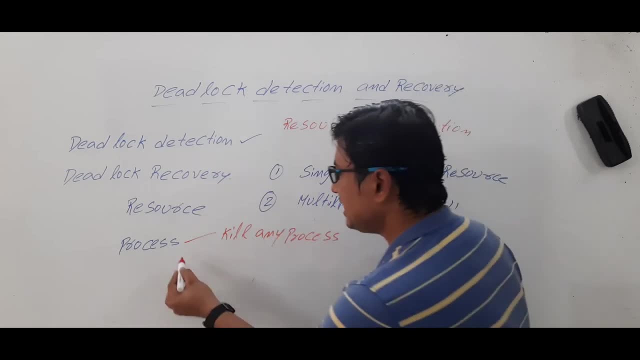 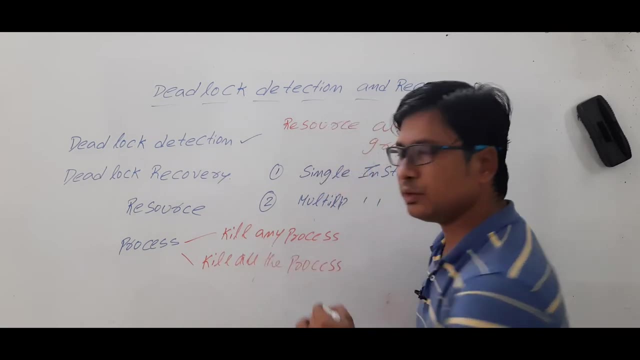 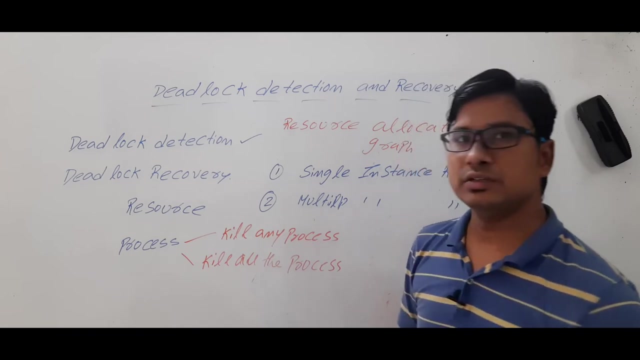 Kill any one process or kill all the process. Is it clear? Are you able to understand it or not? Either kill any one process or kill all the process to recover from the deadlock. Is it clear? Now, coming to the resources: Resources also, we can preempt the resource. 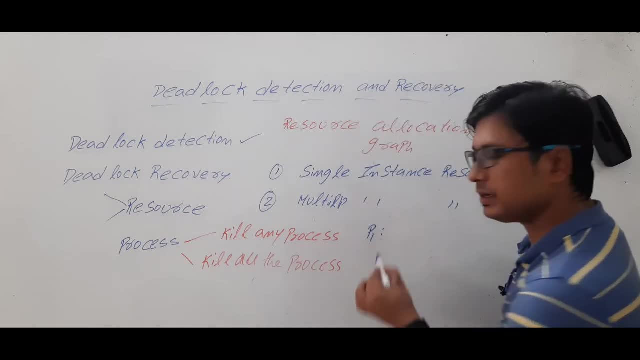 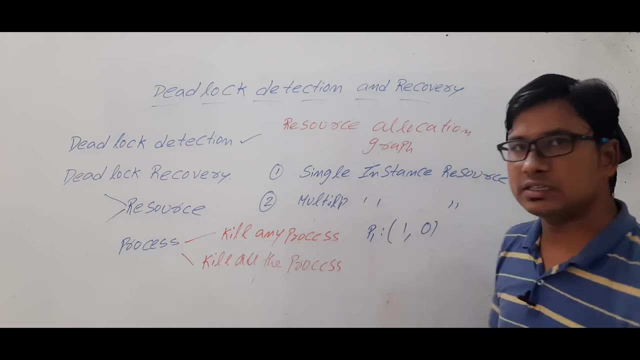 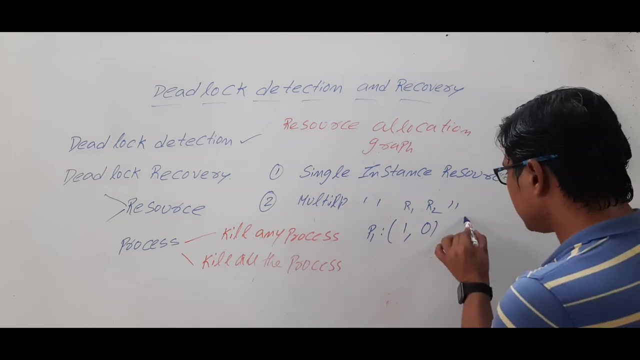 Meaning is that let us take that process, P1. In previous example, the availability is 1 and 0. Meaning is that it has the one instance of resource R1 and it does not have the resource R2. And it is requesting for the resource R2.. 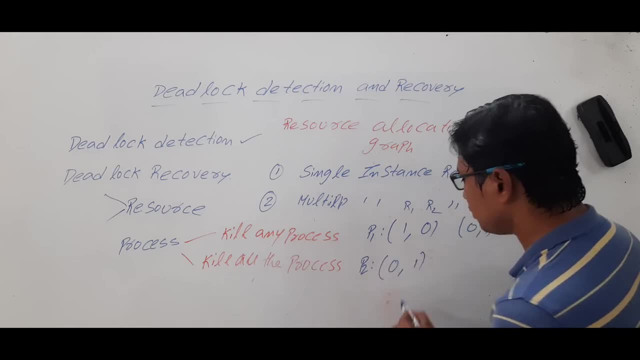 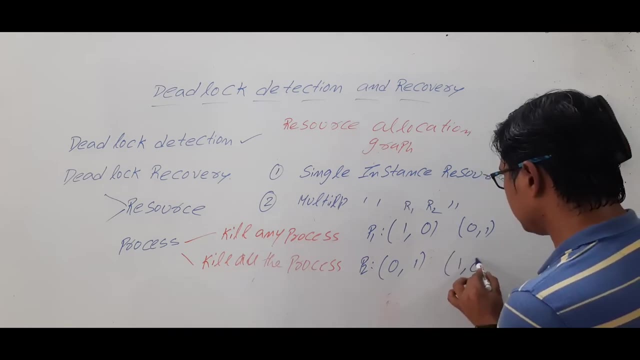 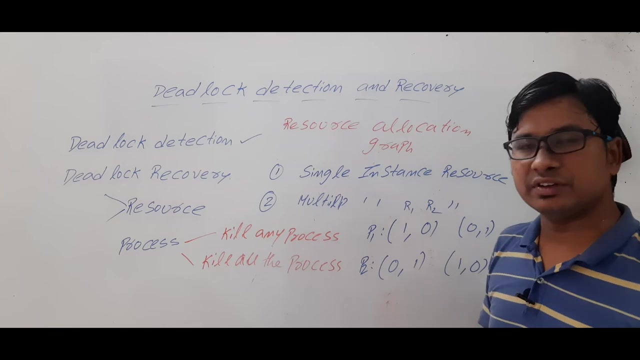 Similarly, process P2, availability is 0, 1.. It does not have the resource R1, but it has the resource R2.. And it is request is also 1, 0.. Now there is a deadlock Because process P1 has resource R1 and requesting for the resource R2.. 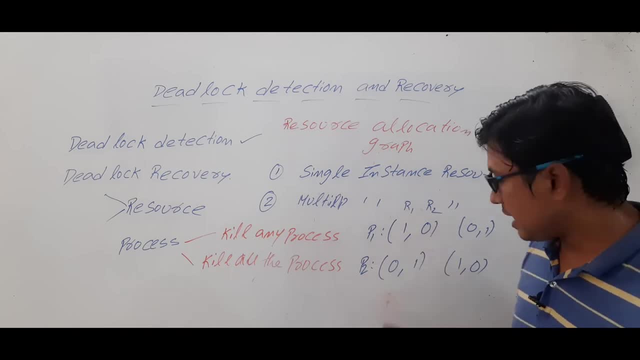 Process P2 is requesting for the resource R1 and it has the resource R2.. Now process P1 can complete the task when it has one instance of resource R1 and one instance of resource R2.. Similarly, process P2 can complete its task when it has one instance of resource R1 and one instance of resource R2.. 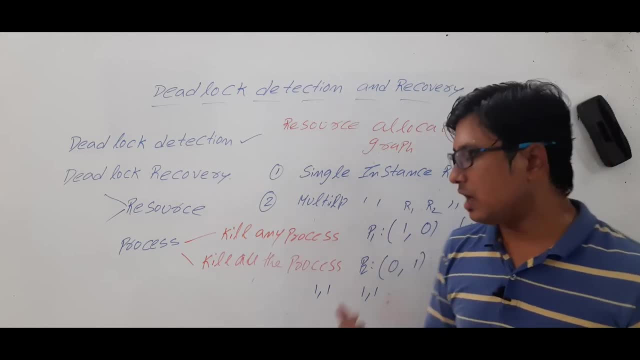 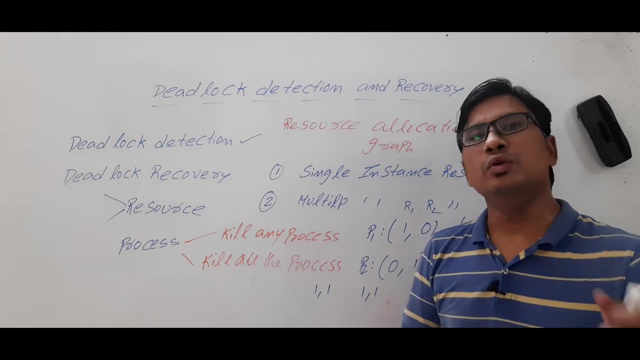 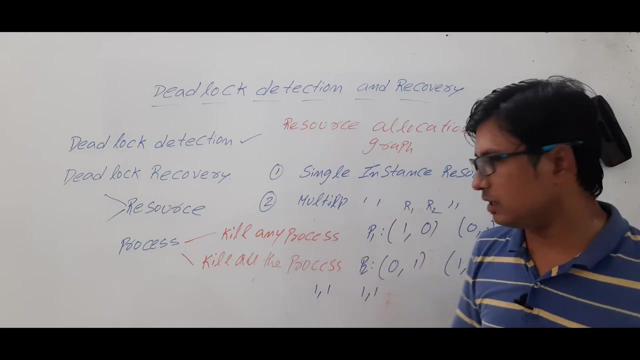 Now both the process are waiting for other process to release the resources, so that leads to a deadlock. so now, what is meant by no preemption? you cannot, the CPU cannot, preempt the resources from the process, is it clear? but when it comes to the preemption, if we use the strategy, 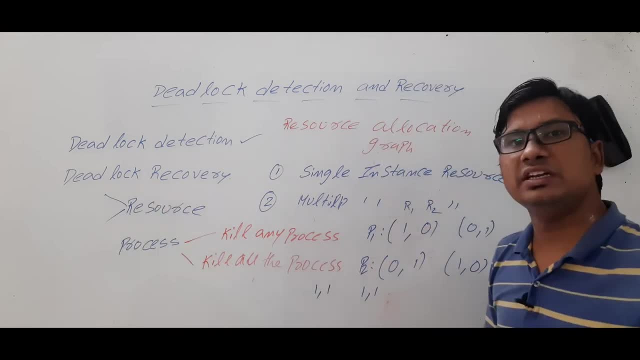 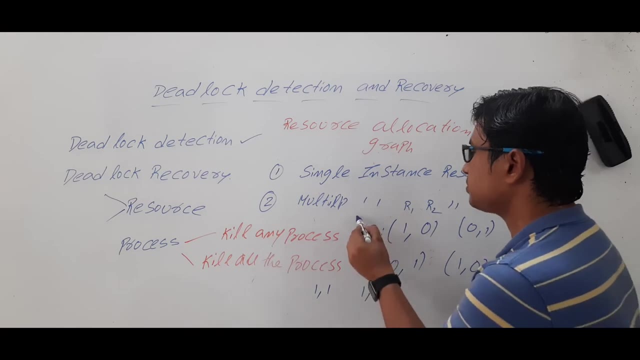 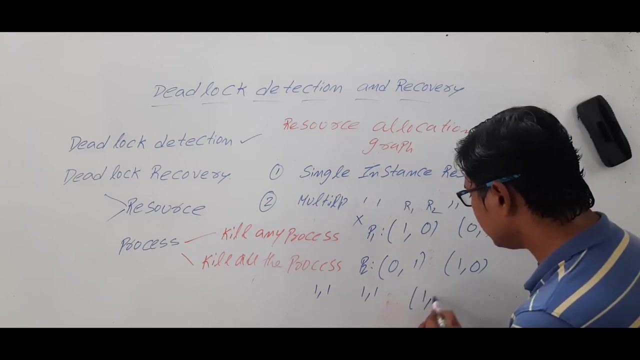 called preempt the resources. meaning is that the CPU is forcefully taking the resource R1 from the process P1. is it clear? if let's take their process, P1 was preempted, then what will be the current availability? current availability will be 1: 0 and, right or wrong, previously availability is 0: 0. we don't have either.